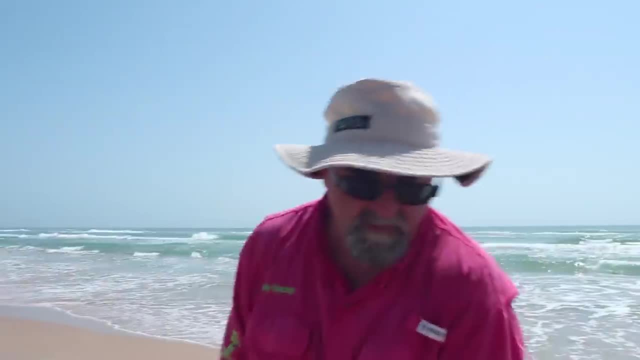 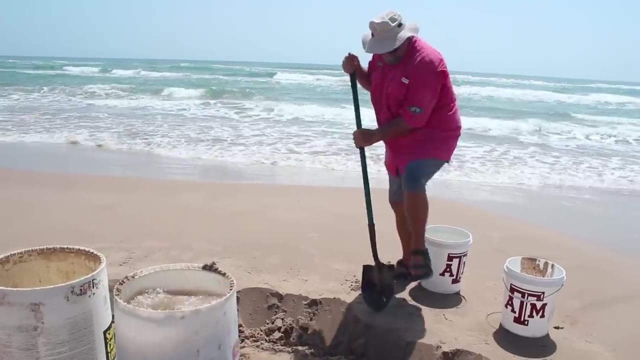 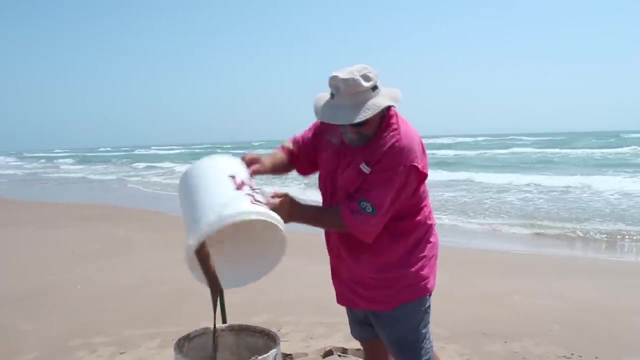 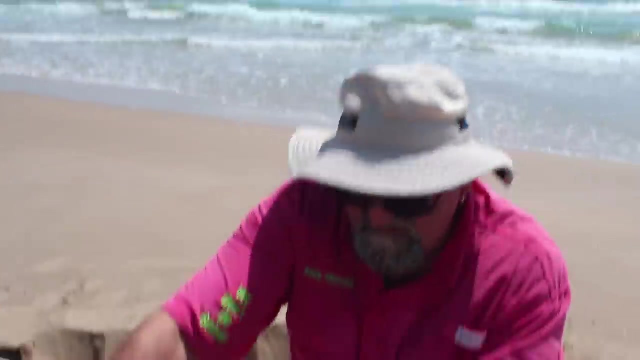 we want to add sand to water, always try not to do it the other way around. it just doesn't work. when these buckets are full of water, we shake them and we tap them. you can see the air bubbles coming out on the top of the sand. we don't want the air mixed with the sand and water, because it 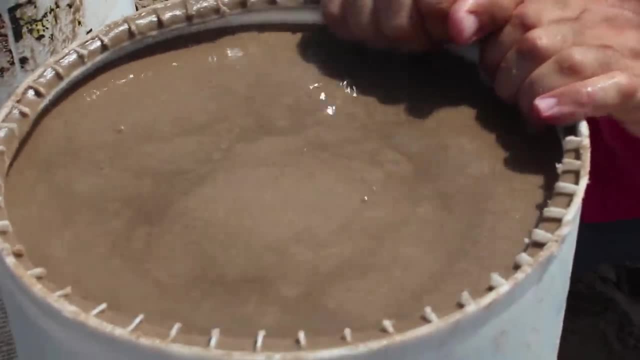 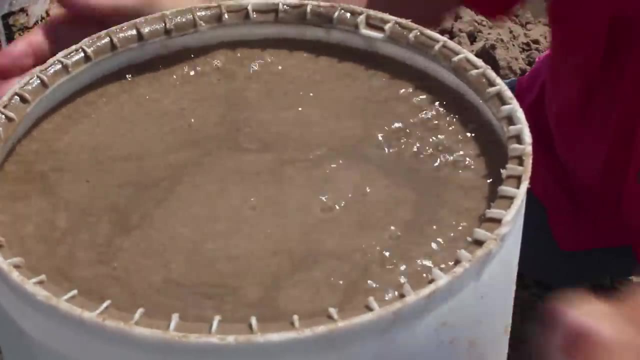 makes it weaker. we want it to be stronger, so we vibrate or tap the bucket to get all the air out. okay, so we've got our two larger buckets ready and we're going to put them in the bucket. now we're going to go ahead and get the air out of them. 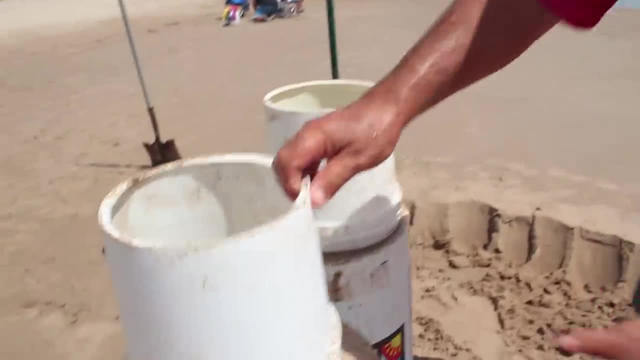 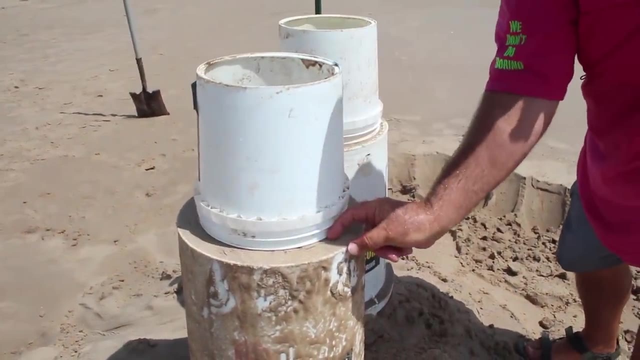 filled. now we're going to add our smaller buckets to the top. now one of the things you can do is, when you look at the top of the, the top of this bucket, you could put the smaller one right in the middle, but that leaves you only a thin gap to put any details we like to offset, which means we like. 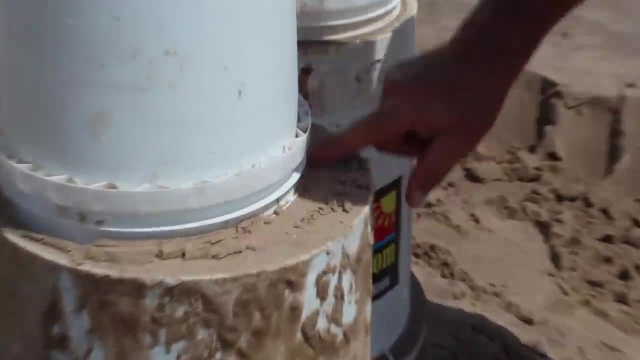 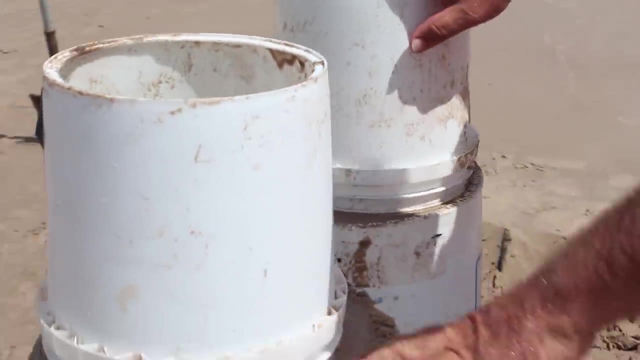 to push that bucket back, to give ourselves a wider distance here, and it doesn't matter about the other side. and then on this one, we like to do it on the other side. so this one's got the wide gap this side. this one's got the wide gap this side. it means that our stairs and any details 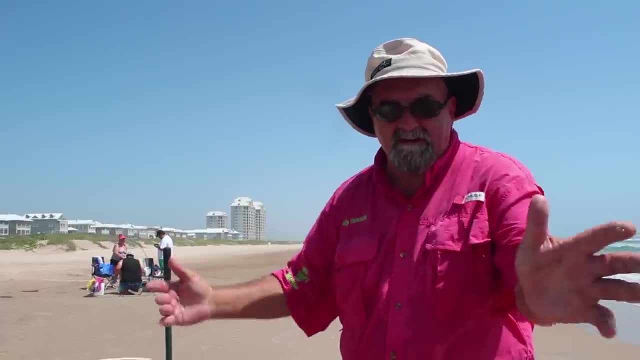 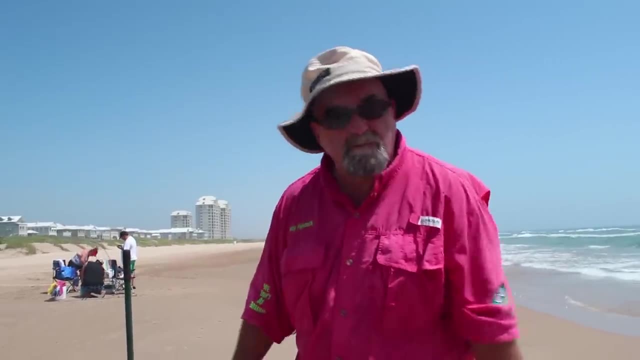 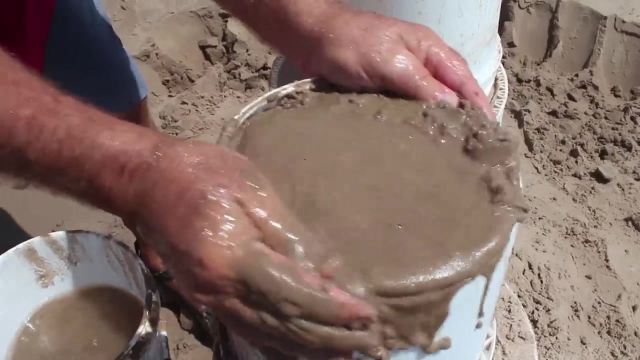 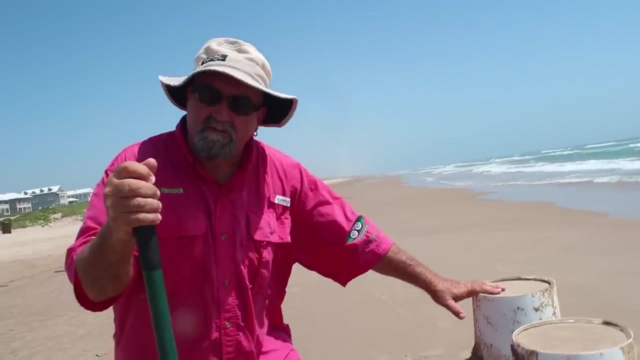 we want can move through the castle from one side to the other. it gives us a lot more interest, creates more details and just looks better. we don't do straight. that's because we don't do boring. we've got these two top buckets full and we're going to pop all the forms at once and then we're. 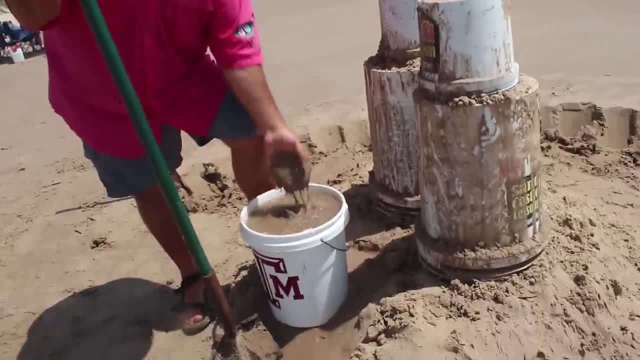 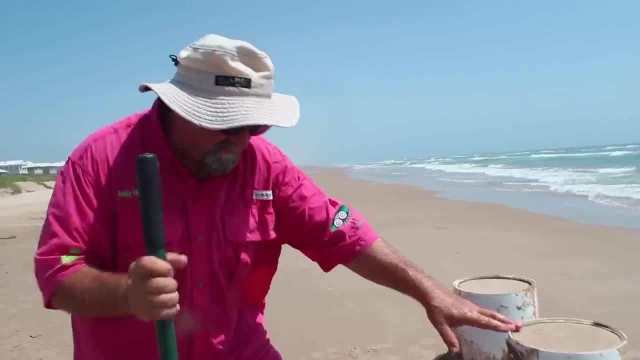 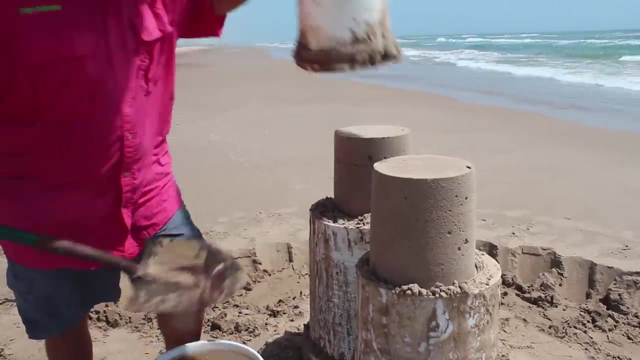 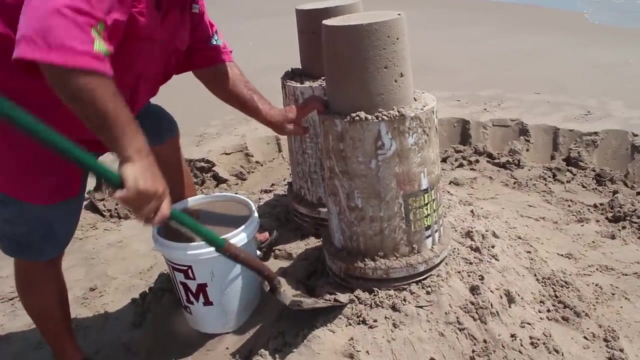 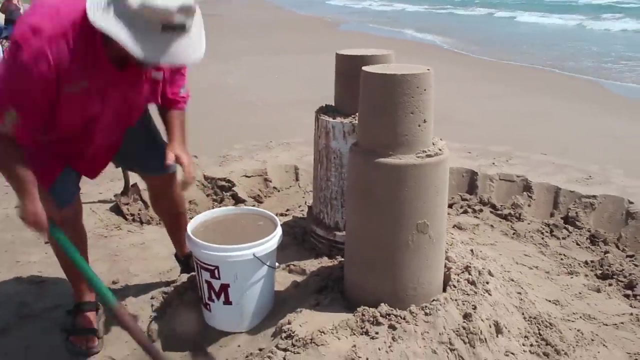 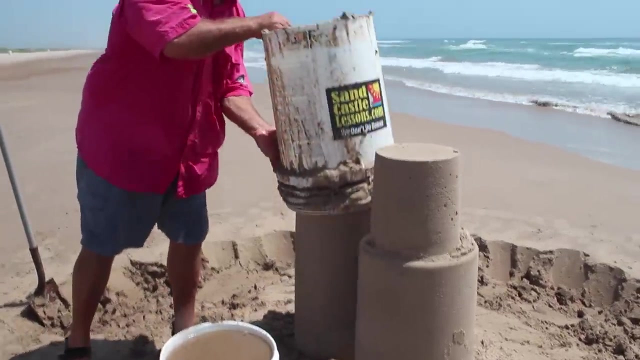 going to fill the gap between with wet sand hand. okay, we've got a bucket prepared here and we're going to fill this gap in between, but first we have to lift these off, and what's made that easier is the WD-40. as you can see, it makes it a really, really quick process and we don't have